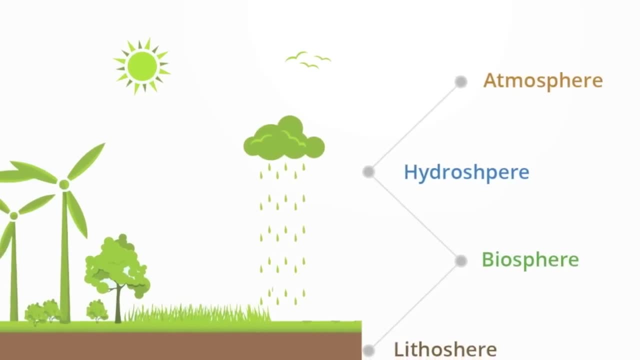 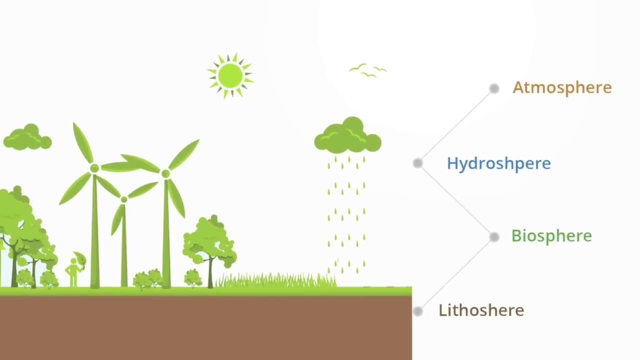 composed of. Thus, the atmosphere is composed of gases, the hydrosphere of liquid water and the lithosphere of solid materials. Added to this is the biosphere, which is a sum total of all biological material and processes. Within each sphere, a process called a cycle takes place. 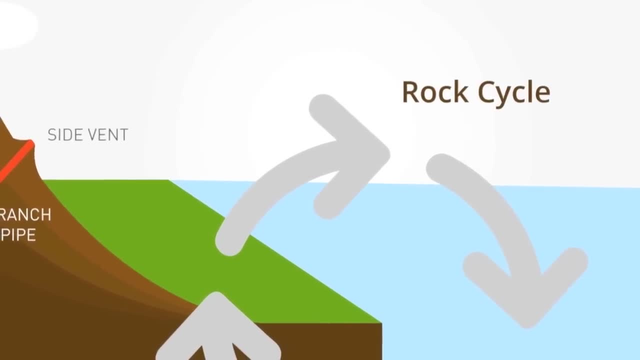 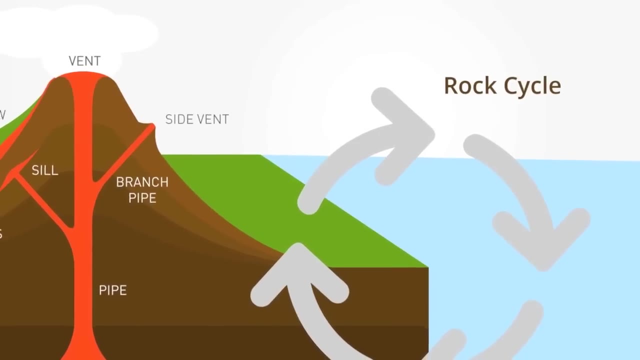 For example, in the lithosphere we have the rock cycle, driven by the thermal energy within Earth's interior that releases minerals through ocean ridges and volcanoes that are weathered as they cycle through the Earth's crust and are eventually subducted, returning to their 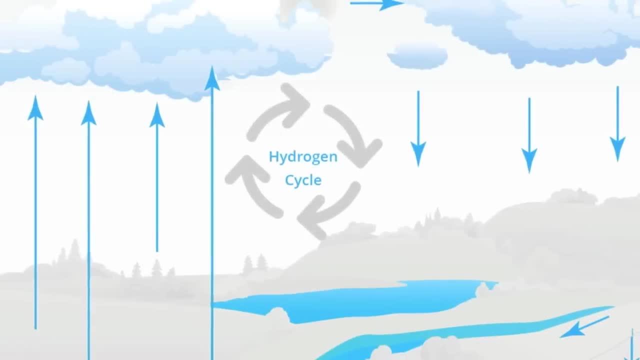 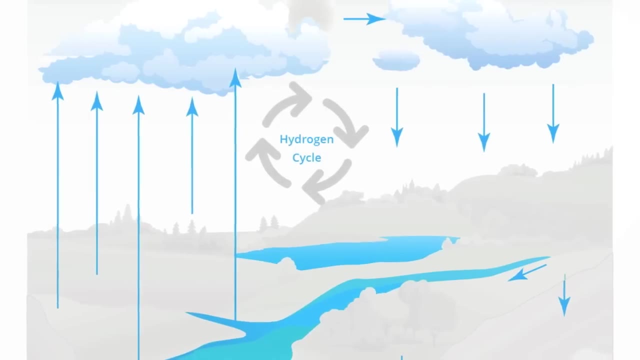 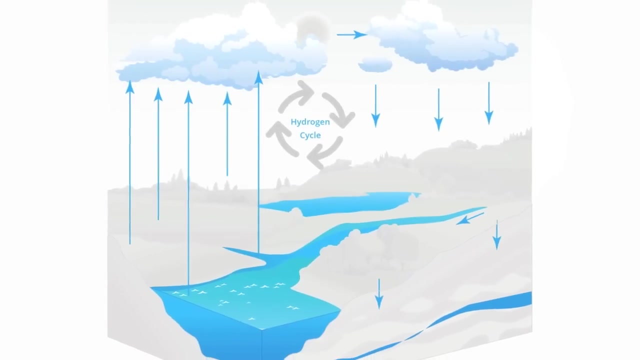 origin. The hydro cycle, driven by the thermal energy of the Sun, cycles water between the Earth's surface and atmosphere through the process of evaporation, condensation and precipitation. This process helps to distribute moisture to support ecosystems at a variety of locations. 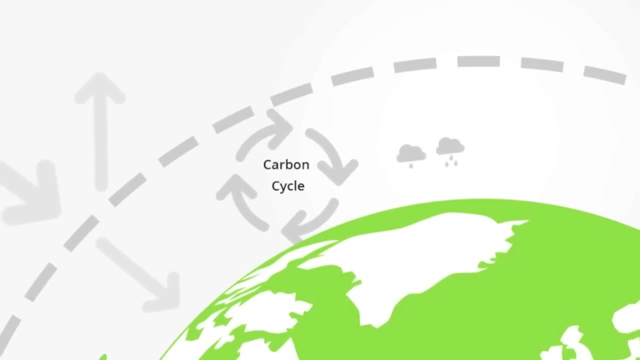 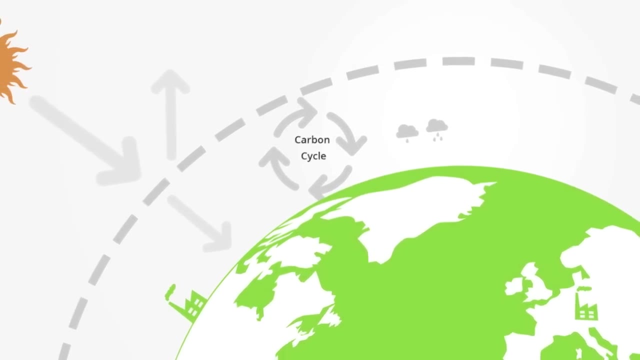 The atmosphere is a layer of gases surrounding the planet that is held in place by gravity. It is the primary vehicle of temperature and climate regulation through the cycle of carbon in and out of the atmosphere, where it functions through the greenhouse effect to trap the 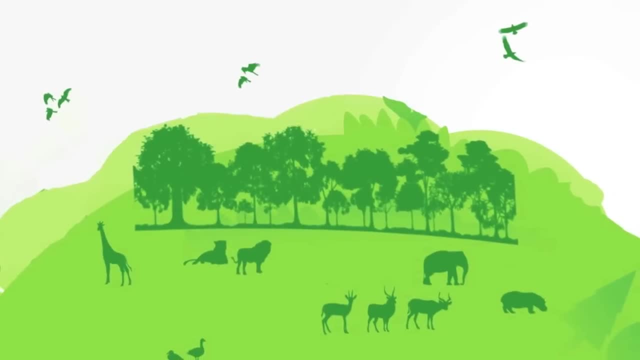 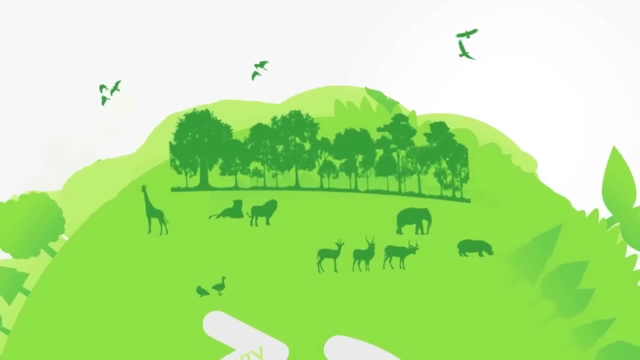 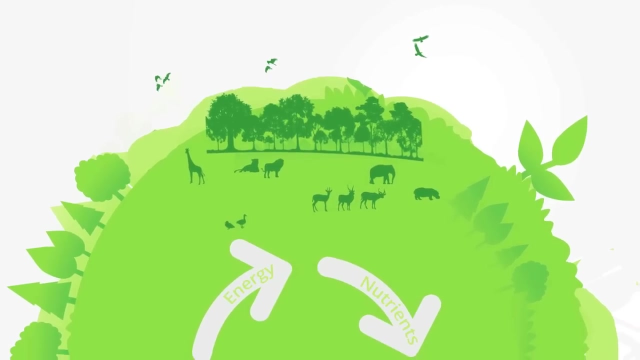 Sun's heat. The biosphere is the relatively three-dimensional atmosphere of the Earth. It is a very thin layer of Earth's surface that supports all biological activity. The biosphere is a system also characterized by the continuous cycle of material and energy in the form of the flow of solar energy and nutrient-mineral cycles. 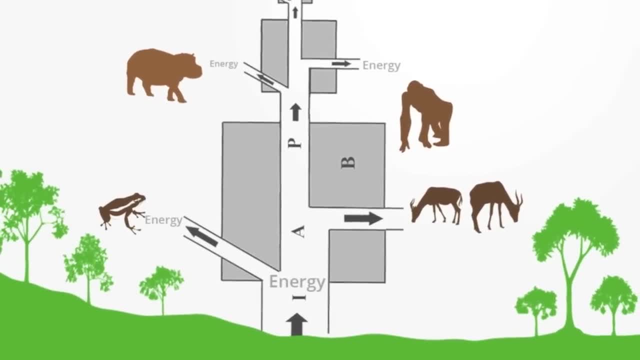 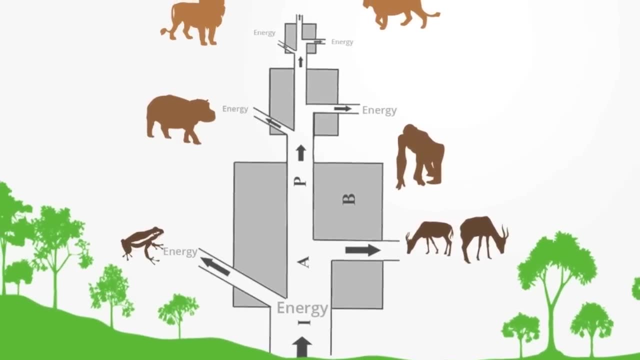 Solar energy flows through the biosphere along a unidirectional path, as the Sun's energy is inputted through plant photosynthesis and processed up through what are called trophic levels, from primary producers to herbivores and on to predators and apex predators. 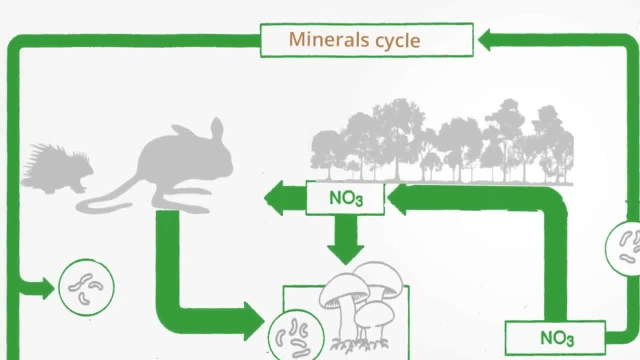 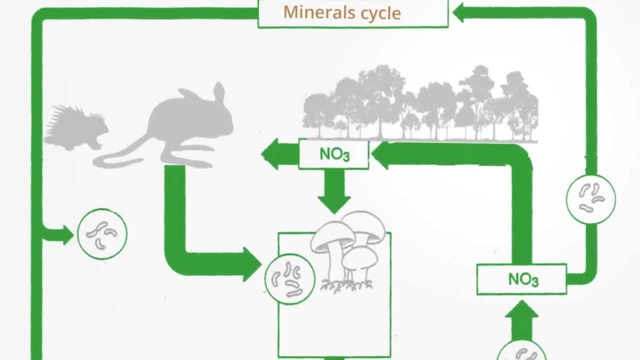 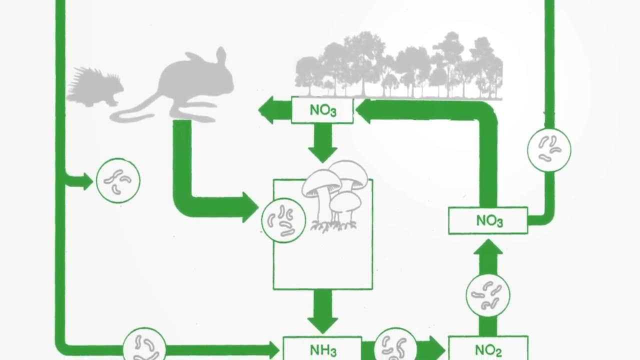 Alongside the flow of energy through food webs is the cycle of mineral nutrients, the core substances required for the construction of biological material and processes. Carbon, water, oxygen and nitrogen have been continuously cycled through the biosphere from one generation to the next for billions of years. 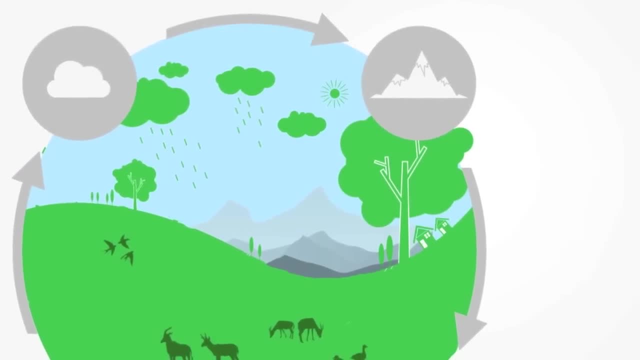 These different spheres interact to create a unique state or ecosystem. An ecosystem is the combination of a community of biological organisms and a community of biological organisms. These different spheres interact to create a unique state or ecosystem. An ecosystem is the combination of a community of biological organisms and a community of